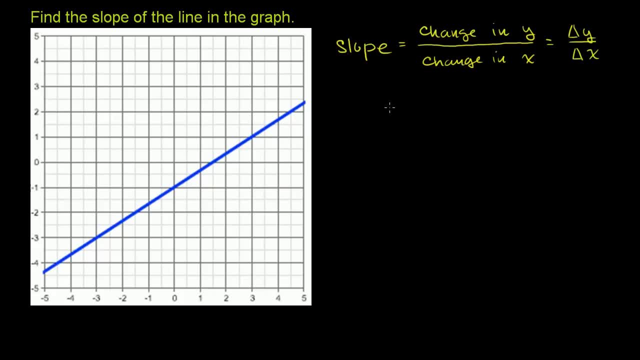 So let's see what this change in y is for any change in x. So let's start at some point that seems pretty reasonable to remember. Read from this table, right here, from this graph. So let's see, We're starting here. 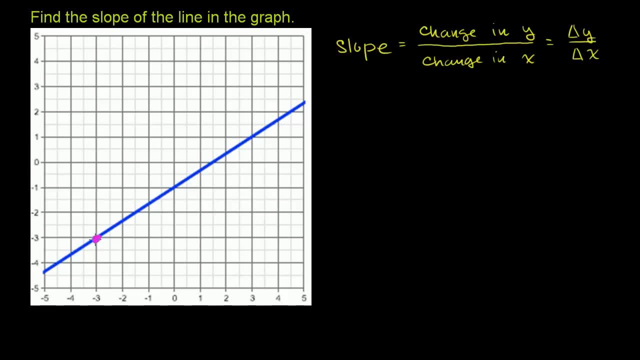 Let me do it in a more vibrant color. So let's say we start at that point right there And we want to go to another point. that's pretty straightforward to read, So we can move to that point right there. We can literally pick any two points on this line. 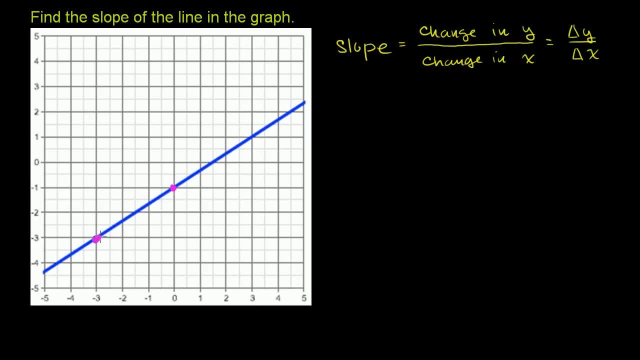 I'm just picking ones that are at nice integer coordinates, so it's easy to read. So what is the change in y and what is the change in x? So first let's look at the change in x. So if we go from there to there, we're 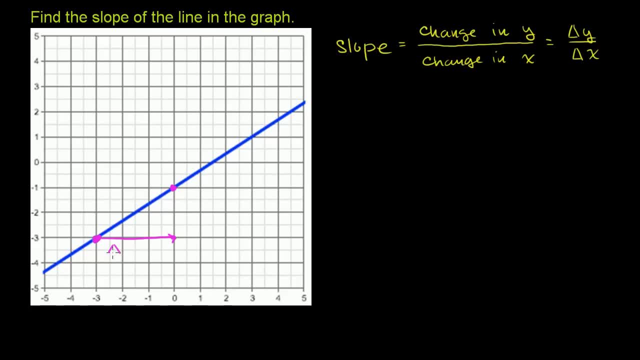 right to there. what is the change in x? My change in x is equal to what? Well, I could just count it out. I went one step, two steps, three steps. My change in x is 3.. And you could even see it from the x values. 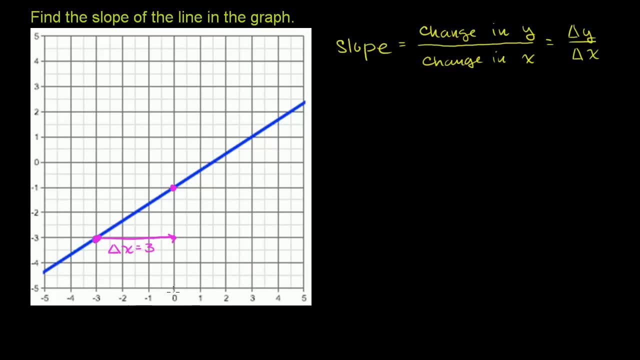 If I go from negative 3 to 0,, I went up by 3.. So my change in x is 3.. So let me write this Change in x: delta x is equal to 3.. And what's my change in y? 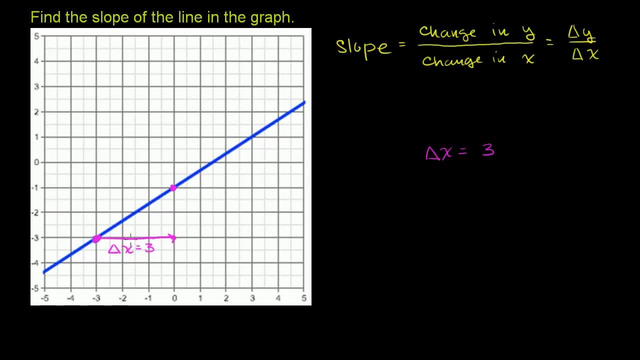 Well, my change in y: I'm going from negative 3 up to negative 1.. Or you could just say 1, 2.. So my change in y is equal to positive 2.. Let me write that down. Change in y is equal to 2.. 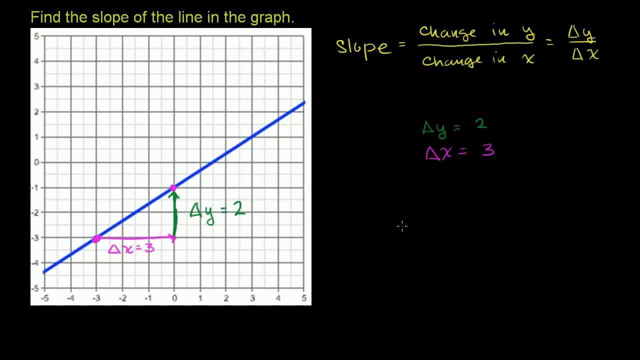 So what is my change in y for a change in x? Well, when my change in x was 3, my change in y is 2.. So this is my change in y. So what is my change in y for a change in x? 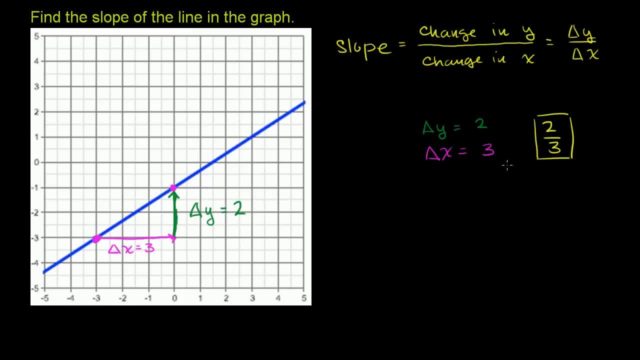 This is my slope And one thing I want to do. I want to show you that I could have really picked any two points here. Let's say I didn't pick those two points. Let me pick some other points And I'll even go in a different direction. 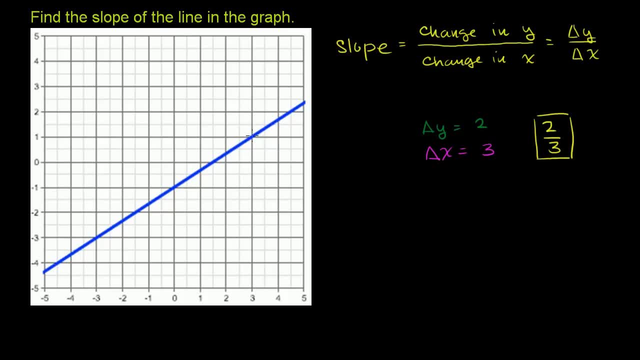 And I want to show you that you're going to get the same answer. Let's say, I viewed this as my starting point And I want to go all the way over there. So what is my? well, let's think about the change in y first. 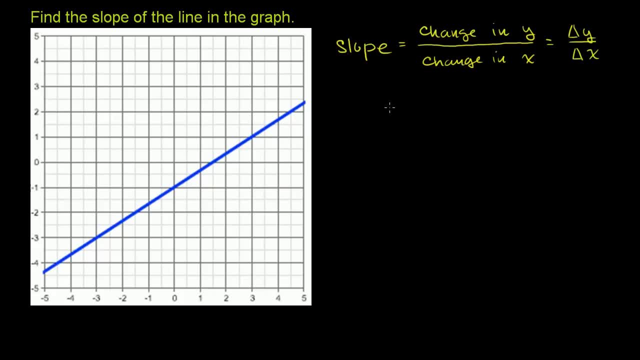 So let's see what this change in y is for any change in x. So let's start at some point that seems pretty reasonable to remember. Read from this table, right here, from this graph. So let's see, We're starting here. 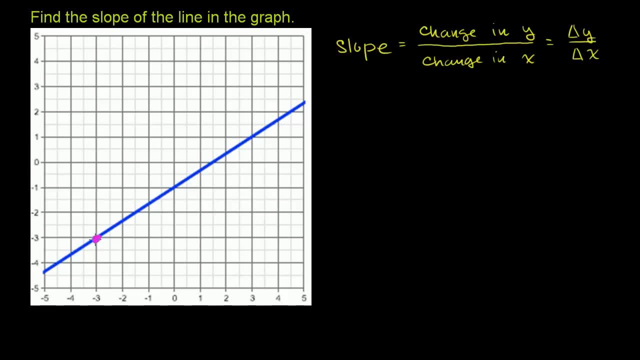 Let me do it in a more vibrant color. So let's say we start at that point right there And we want to go to another point. that's pretty straightforward to read, So we can move to that point right there. We can literally pick any two points on this line. 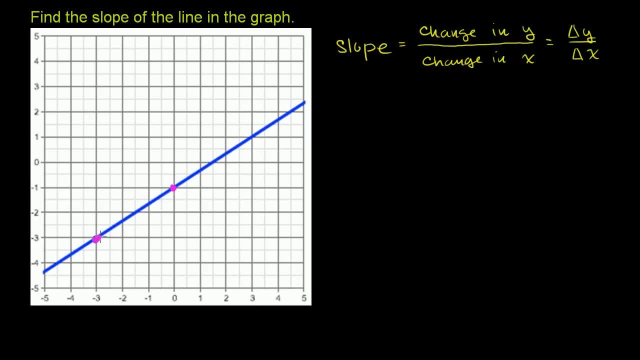 I'm just picking ones that are at nice integer coordinates, so it's easy to read. So what is the change in y and what is the change in x? So first let's look at the change in x. So if we go from there to there, we're 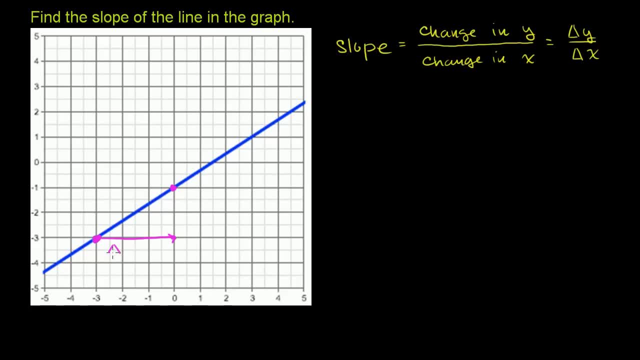 right to there. what is the change in x? My change in x is equal to what? Well, I could just count it out. I went one step, two steps, three steps. My change in x is 3.. And you could even see it from the x values. 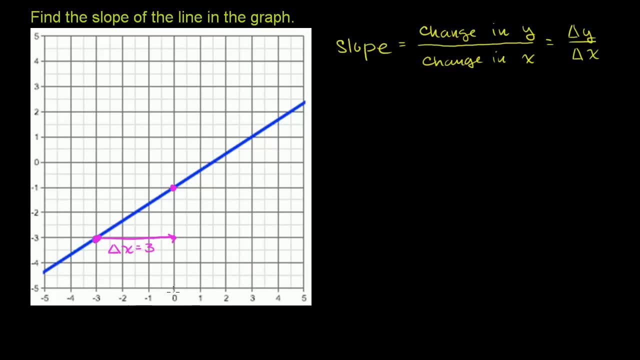 If I go from negative 3 to 0,, I went up by 3.. So my change in x is 3.. So let me write this Change in x: delta x is equal to 3.. And what's my change in y? 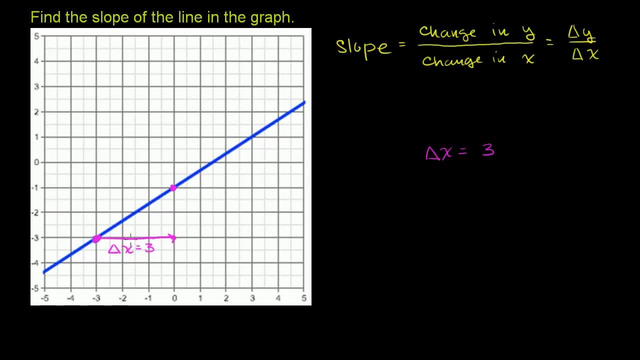 Well, my change in y: I'm going from negative 3 up to negative 1.. Or you could just say 1, 2.. So my change in y is equal to positive 2.. Let me write that down. Change in y is equal to 2.. 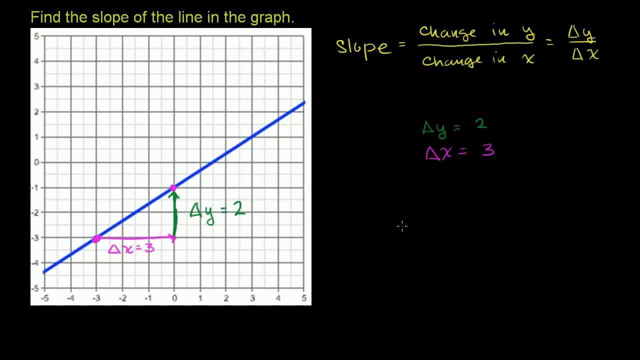 So what is my change in y for a change in x? Well, when my change in x was 3, my change in y is 2.. So this is my change in y. So what is my change in y for a change in x? 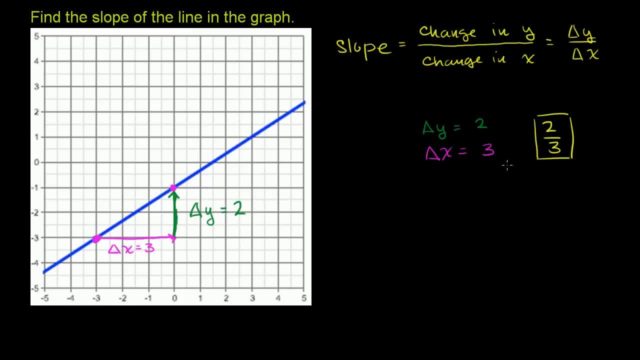 This is my slope And one thing I want to do. I want to show you that I could have really picked any two points here. Let's say I didn't pick those two points. Let me pick some other points And I'll even go in a different direction. 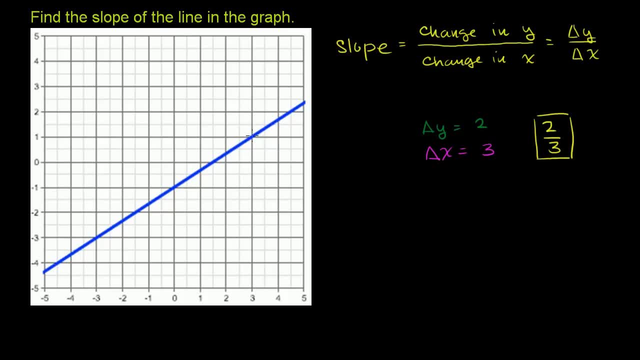 And I want to show you that you're going to get the same answer. Let's say, I viewed this as my starting point And I want to go all the way over there. So what is my? well, let's think about the change in y first. 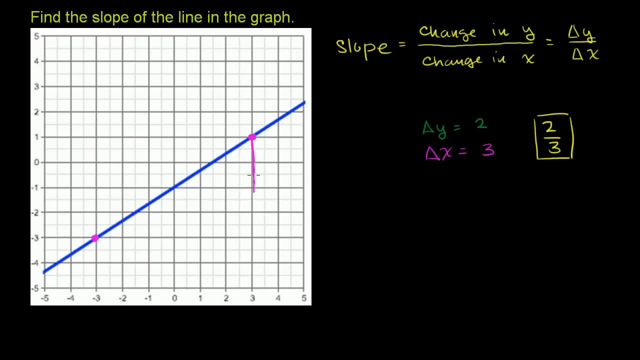 So the change in y. I am going down by how many units: 1,, 2,, 3,, 4 units. So my change in y in this example is negative 4. I went from 1 to negative 3.. 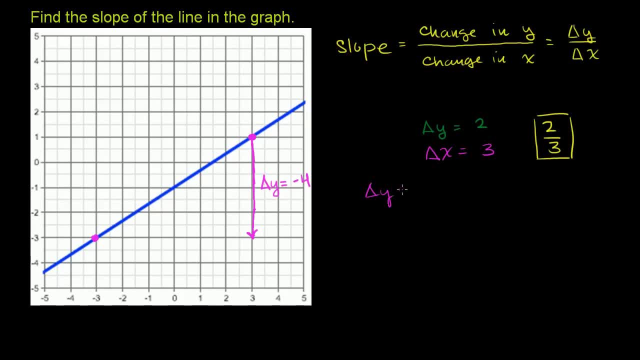 That's negative 4.. That's my change in y. Change in y is equal to negative 4.. Now, what is my change in x? Well, I'm going from this point or from this x value all the way. let me do that in a different color, all. 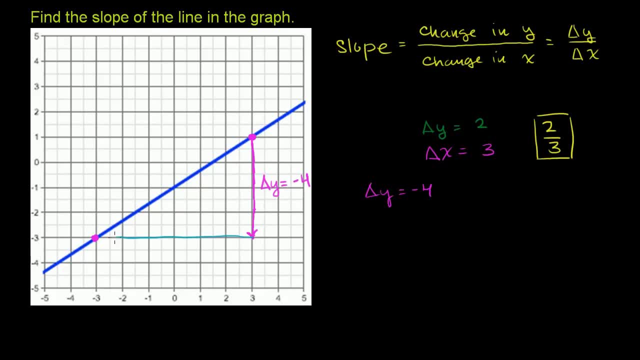 the way, all the way back, like this. So I'm going to the left, so it's going to be a negative change in x And I went 1,, 2,, 3,, 4,, 5, 6 units back. 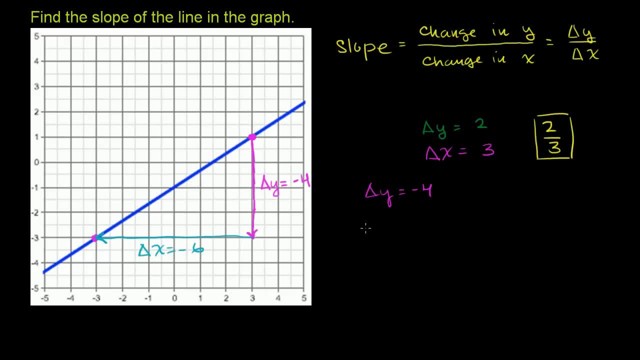 So my change in x is equal to negative 6. Change in x is equal to negative 6. And you could even see. I started at an x is equal to 3. And I went all the way to x is equal to a negative 3.. 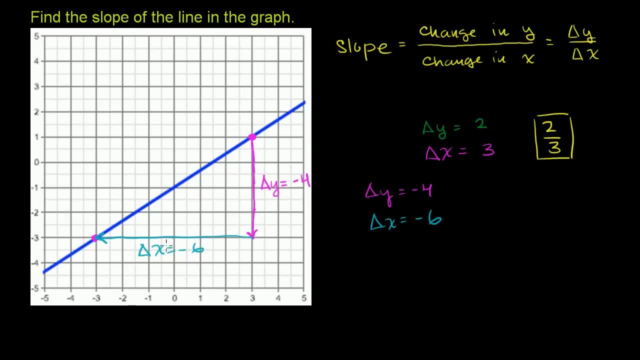 That's a change of negative 6.. I went 6 to the left, or a change of negative 6.. So what is my change in y over change in x? My change in y over change in x is equal to negative 4 over negative 6.. 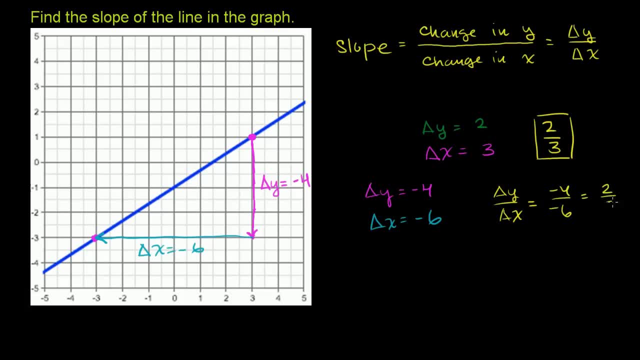 The negatives cancel out. And what's 4 over 6?? Well, that's just 2 over 3.. So it's the same value, You just have to be consistent. If this is my start point, I went down 4,. 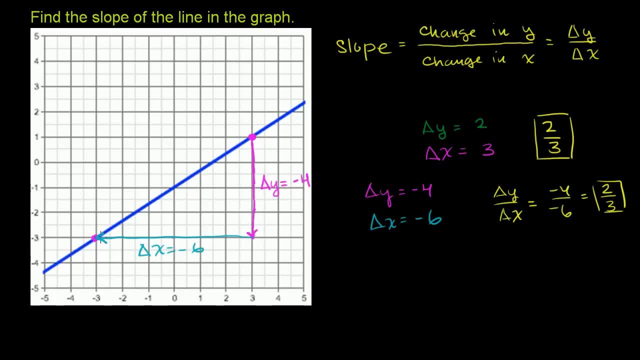 and then I went back 6.. Negative 4 over negative 6. If I viewed this as my starting point, I could say that I went up 4.. So a change in y would be 4. And then my change in x would be 6.. 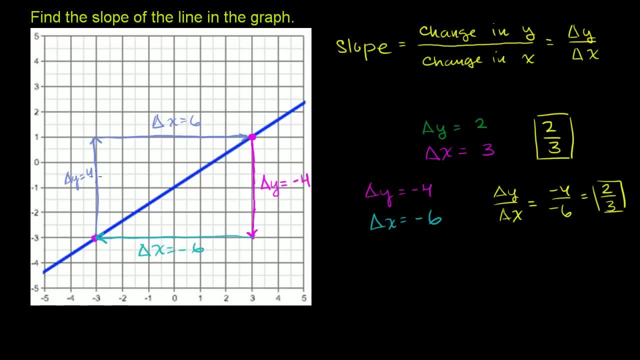 And either way, once again, change in y over change in x is going to be 4 over 6. 2 thirds. So no matter which point you choose, as long as you think about it in a consistent way, you're going to get the same value for slope.